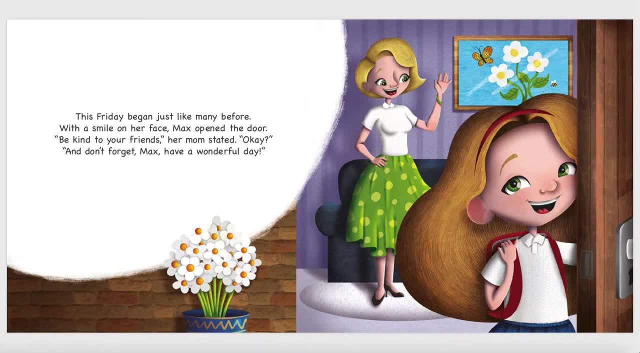 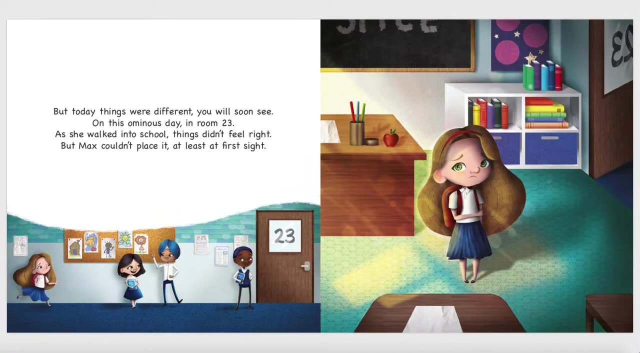 This Friday began just like many before. with a smile on her face, Max opened the door. Be kind to your friends. her mom stated. okay, And don't forget, Max, have a wonderful day. But today's things were different. you will soon see. On this ominous day, in room 23,, 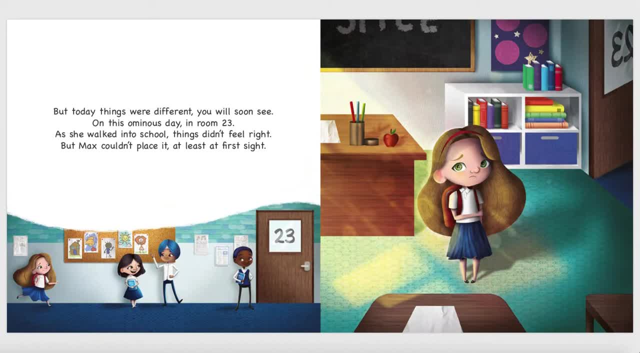 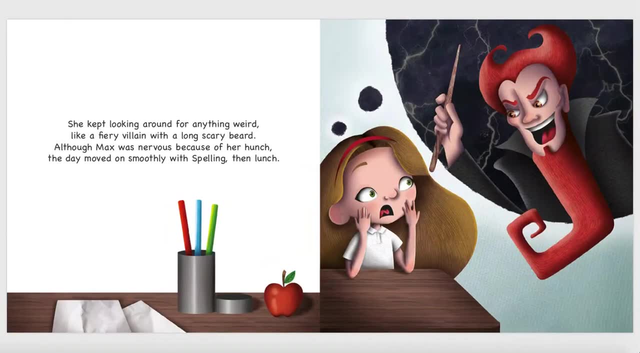 as she walked into school things didn't feel right, but Max couldn't place it, at least at first sight. She kept looking around for anything weird, like a fiery villain with a long, scary beard. Although Max was nervous because of her hunch, the day moved on smoothly with spelling, then lunch. 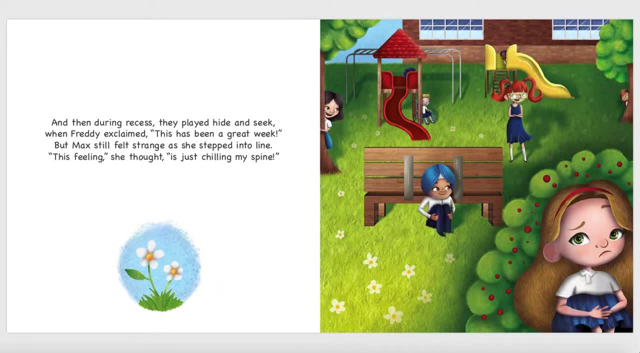 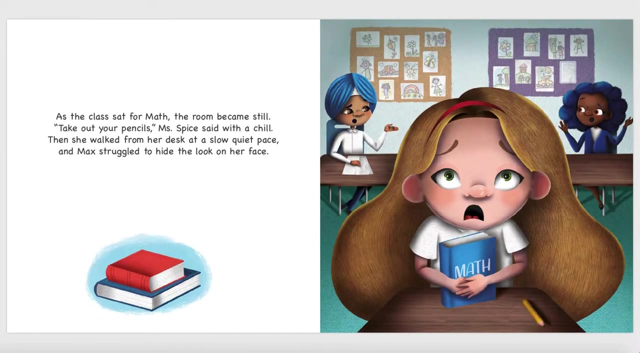 And then during recess they played hide and seek. when Freddie exclaimed: this has been a great week, But Max still felt strange as she stepped into line, This feeling she thought is just chilling my spine. As the class set for math, the room became still Take out your pencils, Ms Spice said with a chill. 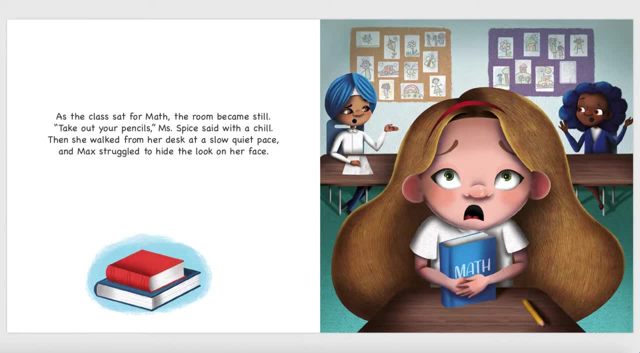 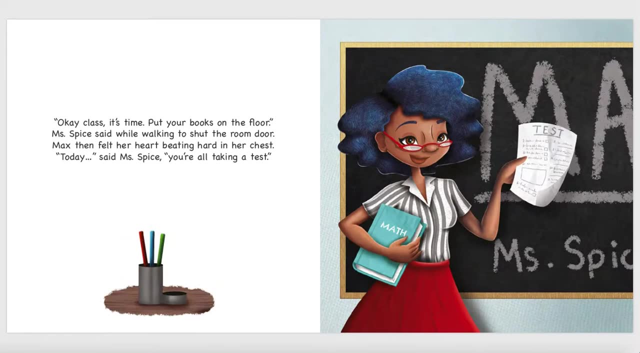 Then she walked from her desk at a slow, quiet pace and Max struggled to hide the look on her face. Okay, class, it's time, put your books on the floor, Ms Spice said. while walking to shut the room door, Max then felt her heart beating hard in her chest. Today, said Ms Spice, 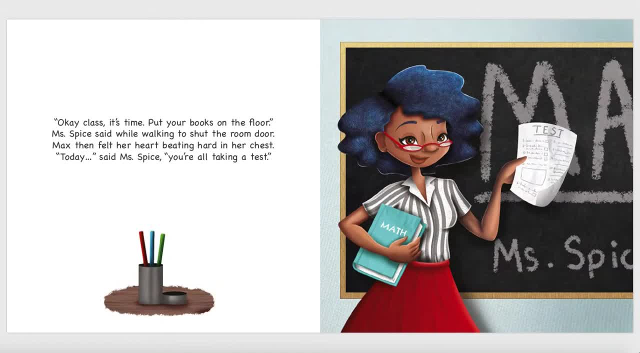 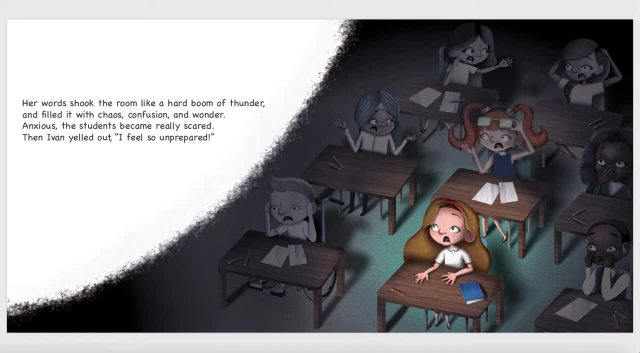 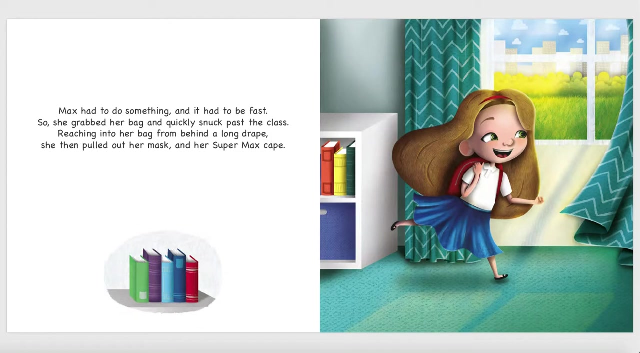 you're all taking a test. Her words shook the room like a hard boom of thunder and filled it with chaos, confusion and wonder. Anxious, the students became really scared. Then Ivan yelled out: I feel so unprepared. Max had to do something and it had to be fast. So she grabbed her bag and quickly snuck past the class. Max had to do something and it had to be fast. So she grabbed her bag and quickly snuck past the class. Max had to do something and it had to be fast, So she grabbed her bag and quickly snuck past the class. 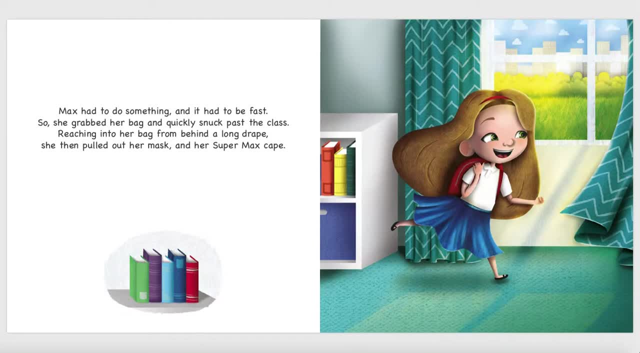 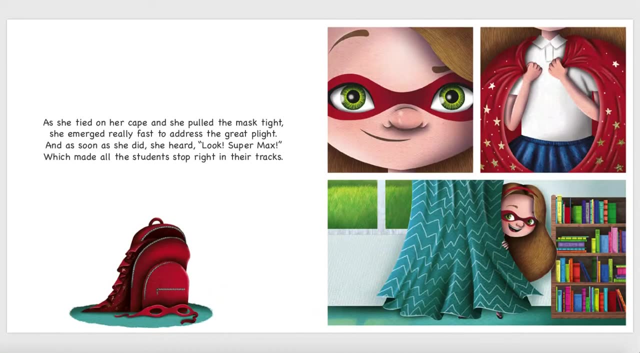 Reaching into her bag from behind a long drape. she then pulled out her mask and her Super Max cape. As she tied on her cape and she pulled the mask tight, she emerged really fast to address the great plight And as soon as she did she heard: look, Super Max. which made all the students stop. 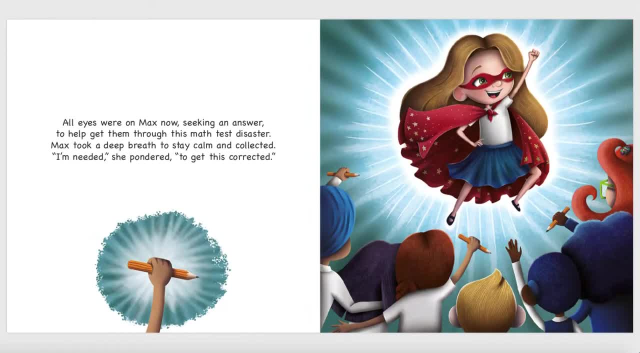 right in their tracks. All eyes were on Max now, Seeking an answer to help get them through this math test disaster. Max took a deep breath to stay calm and collected. I'm needed she pondered to get this corrected. 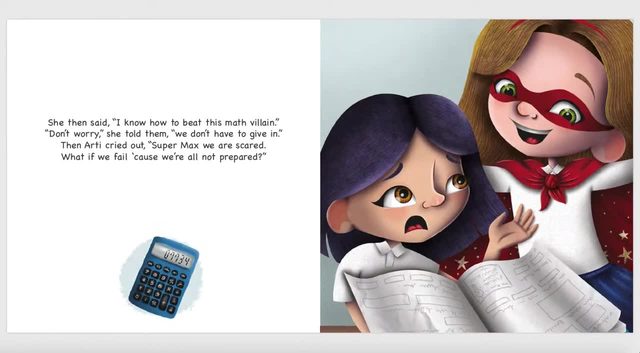 She then said: I know how to beat this math villain, Don't worry. she told them, we don't have to give in. Then Artie cried out: Super Max, we are scared. What if we fail? cuz We're all not prepared. 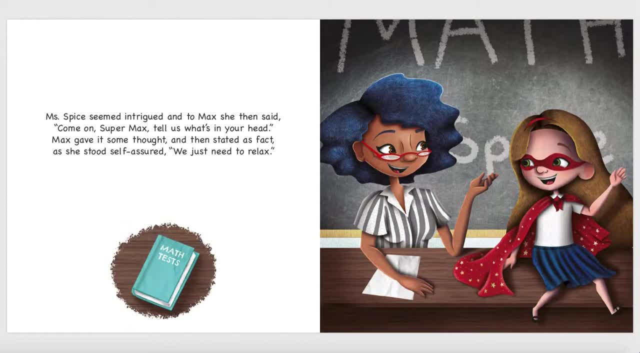 Ms Spice seemed intrigued, and to Max she then said: come on, Super Max, tell us what's in your head. Max gave it some thought and then stated as fact, As she stood self-assured: we just need to relax. 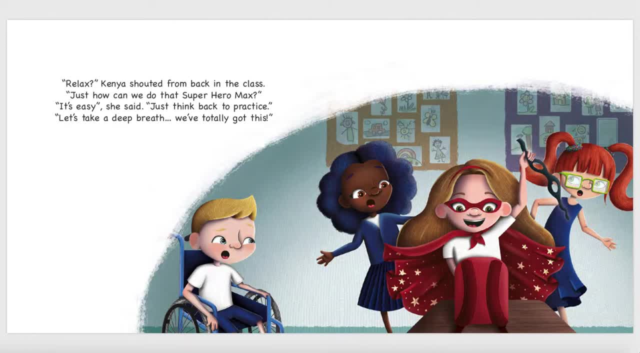 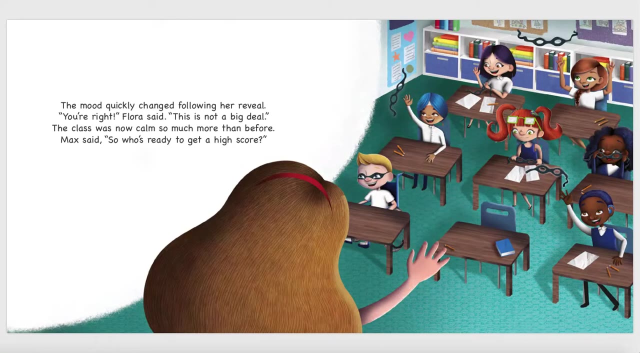 Relax. Kenya shouted from back in the class. Just how can we do that? Super Hero Max, It's easy. she said. Just think back to practice. Let's take a deep breath. We've totally got this. The mood quickly changed following her reveal. You're right. Flora said This is not a big deal. 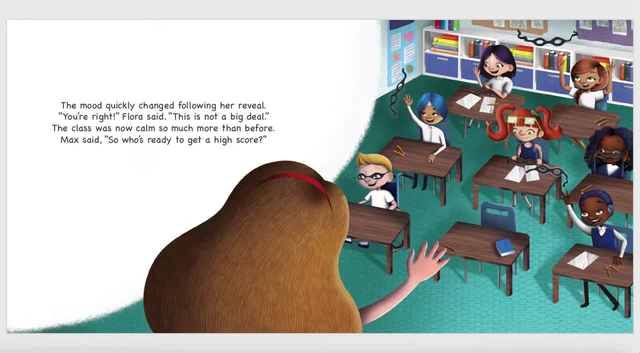 The class was now calm, so much more than before. Max said: So who's ready to get a high score? Her classmates stood up with their eyes open and the teacher was all over the place. Max was not sure what to do, but he was getting the hang of it. She was a little nervous about the math thing. Her classmates stood up with their eyes open. They said: the math is going to be a lot easier than before. Max said so who's ready to get a high score? Max said: who's ready to get a high score? Her classmates stood up with their eyes open. She said: I know how to beat this math villain. 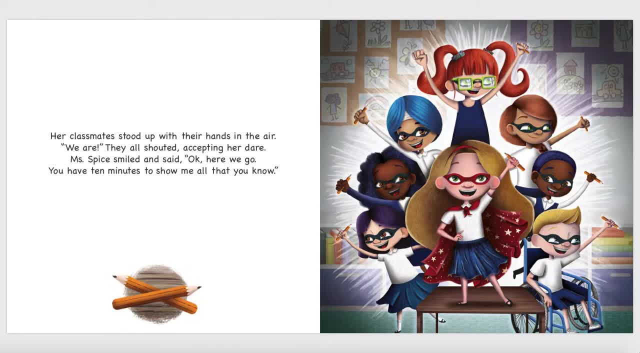 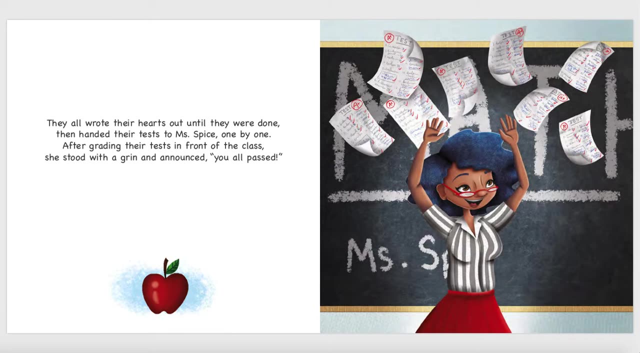 stood up with their hands in the air. We are, they all shouted, accepting her, dare. Miss Spice smiled and said: okay, here we go. You have 10 minutes to show me all that you know. They all wrote their hearts out until they were done, then handed their test to Miss Spice one by one, After grading their 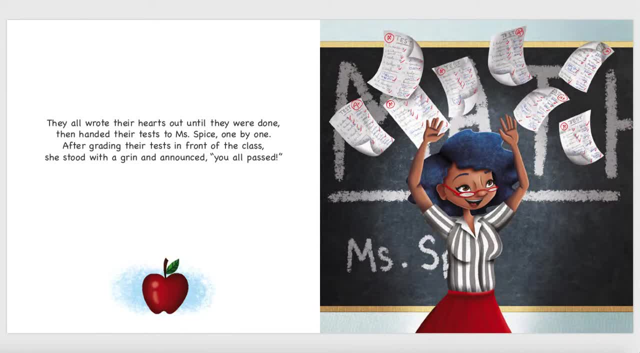 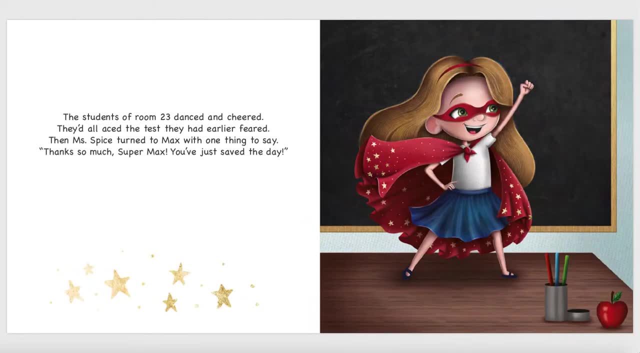 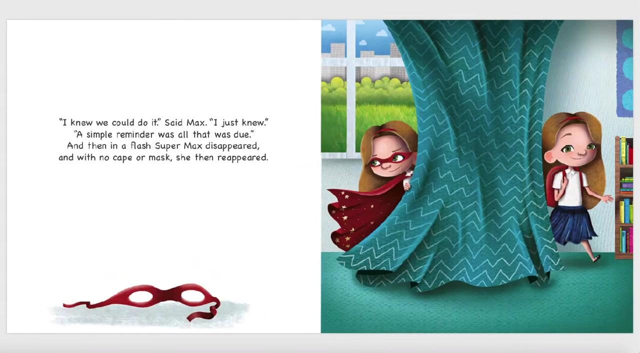 test. in front of the class she stood with a grin and announced: you all passed. The students of room 23 danced and cheered. They'd all aced the test they had earlier feared. Then Miss Spice turned to Max with one thing to say: Thanks. so much, Super Max. You've just saved the day. I knew we could do. 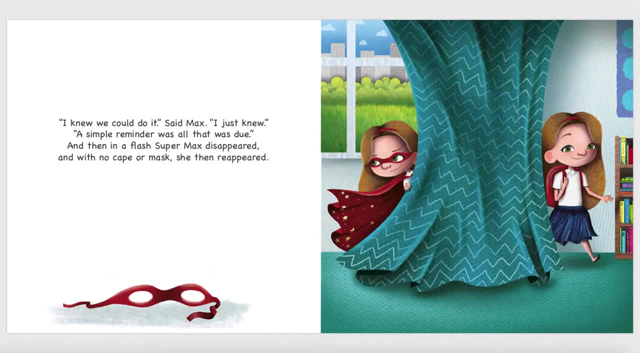 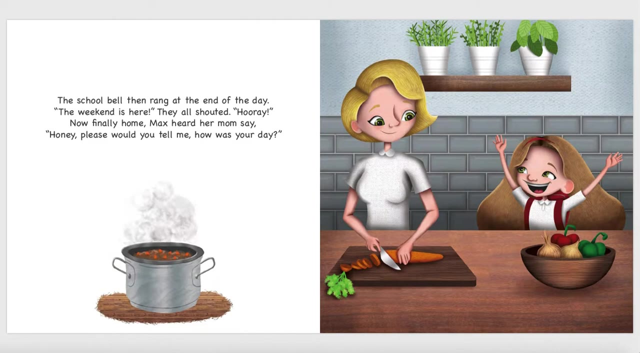 it said Max. I just knew A simple reminder, That was all that was due. And then, in a flash, Super Max disappeared, And with no cape or mask, she then reappeared. The school bell then rang. at the end of the day, The weekend is here. 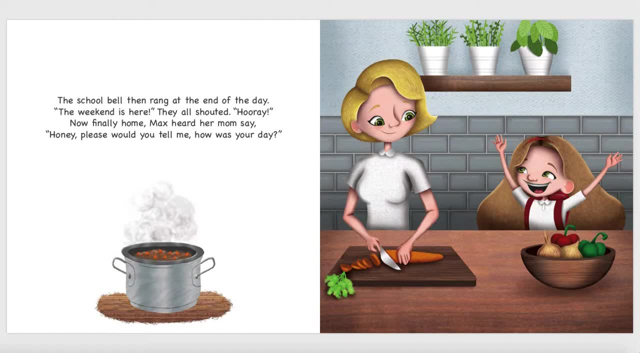 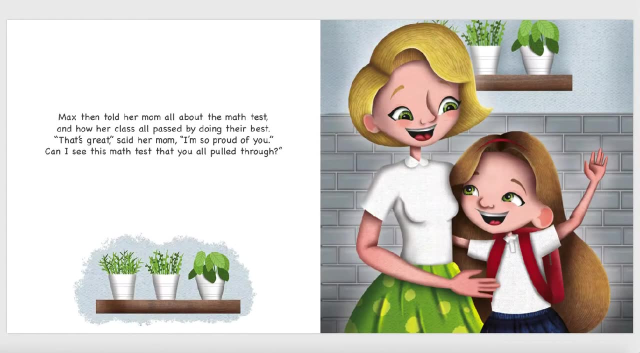 they all shouted: Hooray, Now finally home. Max heard her mom say: honey, please would you tell me how was your day. Max then told her mom all about the math test And how her class all passed by doing their best. That's great, said her mom. I'm so proud of you. 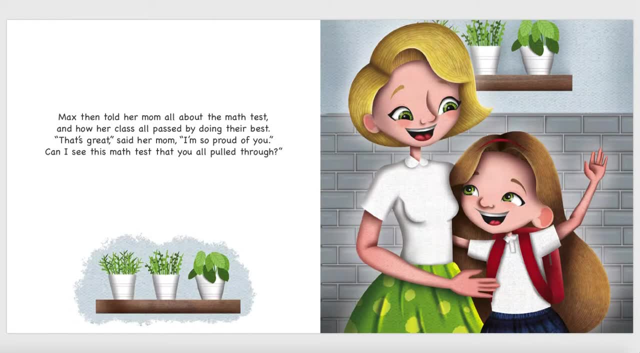 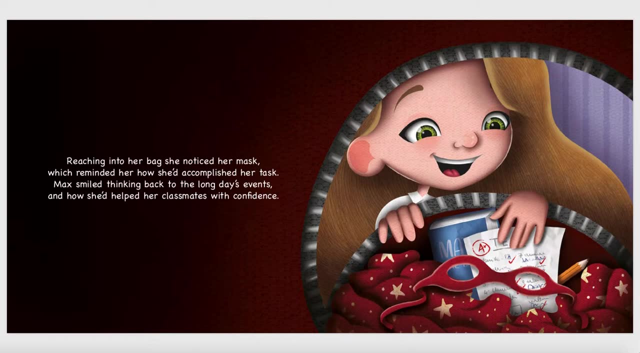 Can I see this math test that you all pulled through? Reaching into her bag, she noticed her mask, which reminded her how she'd accomplished her task. Max smiled, thinking back to the long day's events and how she'd help her classmates. 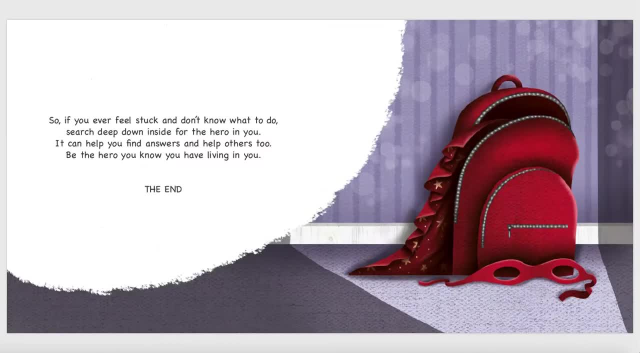 with confidence. So if you ever feel stuck and don't know what to do, search deep down inside for the hero in you. It can help you find answers and help others too, Be the hero you know you have living in you. The end. 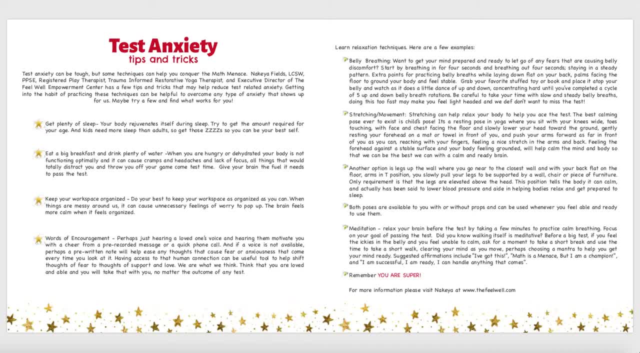 Test Anxiety Tips and Tricks. Test anxiety can be tough, but some techniques can help you overcome it. So if you ever feel stuck and don't know what to do, search deep into your bag. The rest of the tips and tricks help you to conquer the math menace. 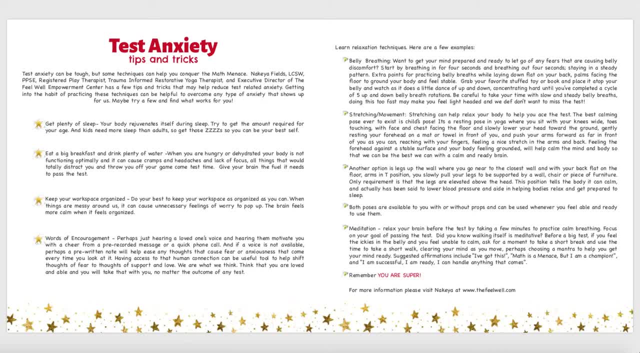 Nakia Fields, LC-SW, PPSE. Registered Play Therapist, Trauma-Informed Restorative Yoga Therapist and Executive Director of the Feel Well Empowerment Center, has a few tips and tricks that may help reduce test-related anxiety: Getting into the habit of practicing these.